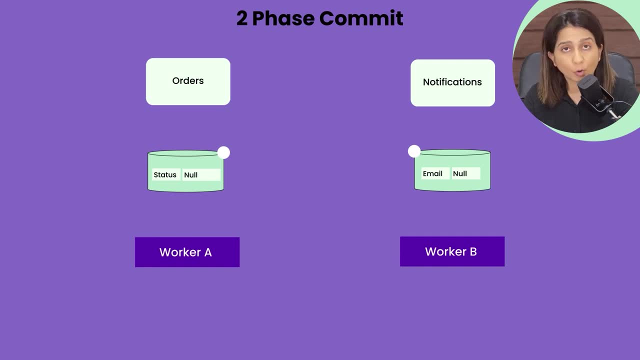 for the sake of simplicity, let's say that you have another service which is called coordinator. what does this service would do? this service will, in first phase, ask both the services if they are ready for a two-phase transaction. okay, in the first step it will ask: are you ready? can you update the state? it will also ask the another service: are you ready, can? 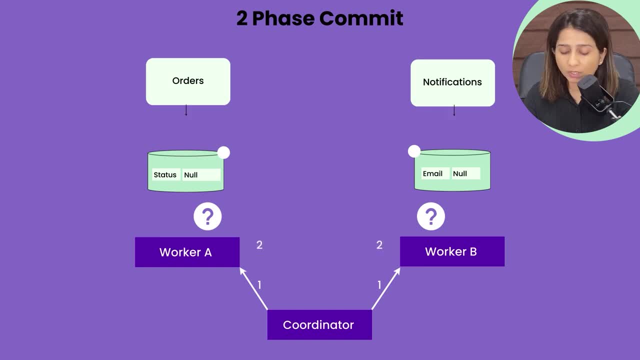 you update the state in the second step. let's say, both the services say, yes, i can update, yes, i can update. so this was the voting phase. both the services said that yes, we can update the state. now in the third step, the commit- actual commit- happens. so this coordinator will say, okay, change. 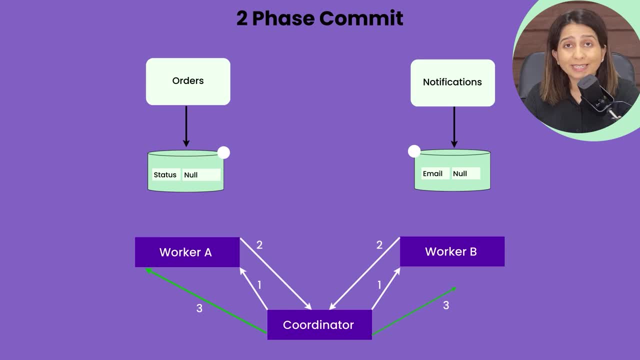 the order state to accepted and change the email state to sent as the fourth step. this order state is accepted and the email state is sent. now how does this happen? after the yes phase, after this second phase, both these services will put a lock on this particular rows and till this transaction completes on both the 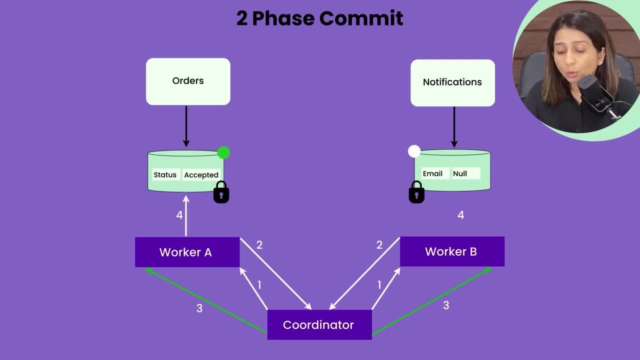 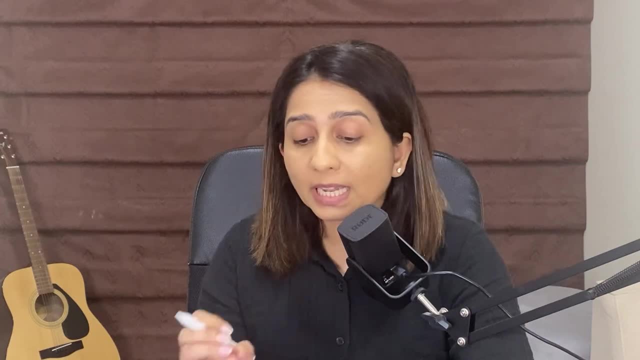 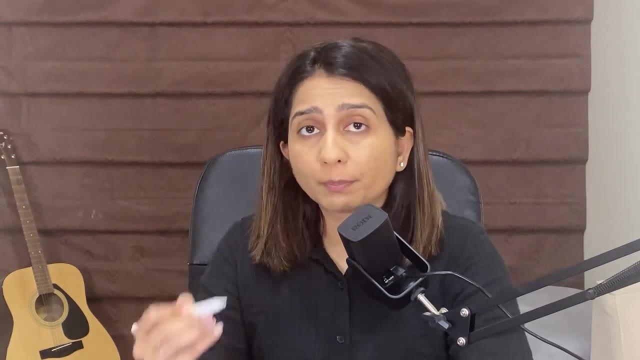 services and this final yes happens from both the services. those rows will stay locked and once that commit happens, both your databases are updated and your transaction is complete. this is known as two phase commit transactions. now it looks simple. if you want to simplify it, you can say that step one and two, here are the vote phases, and three and. 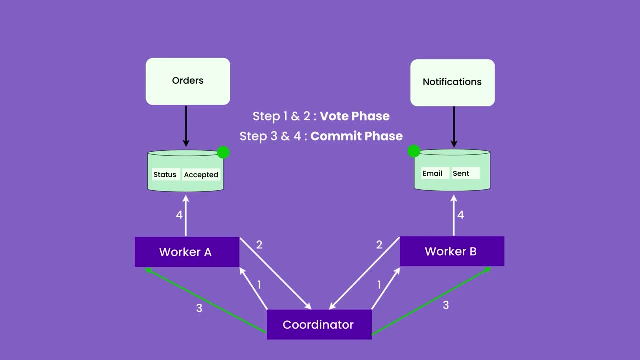 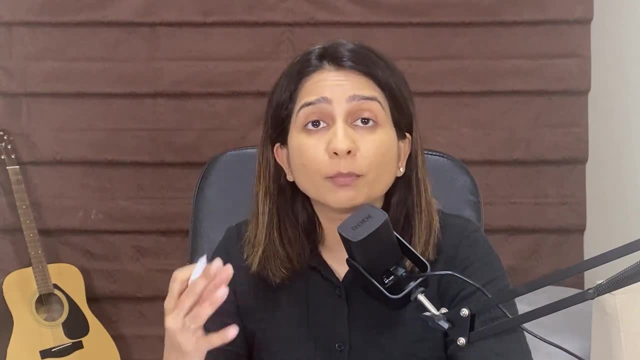 four, here are the commit phases. but the problem comes when you have a very big system. let's say that these databases are huge. these rows that we are talking about sit into the tables which have millions of rows. having log on these rows for multiple transactions will increase the latency of 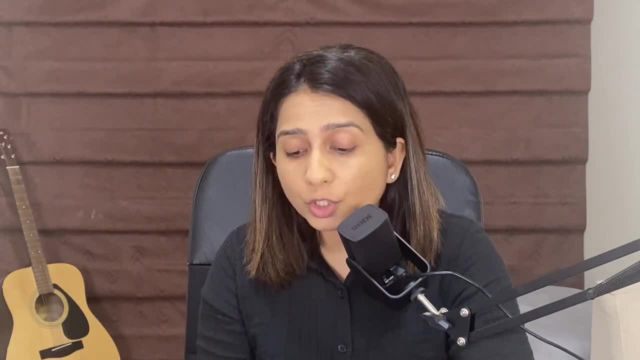 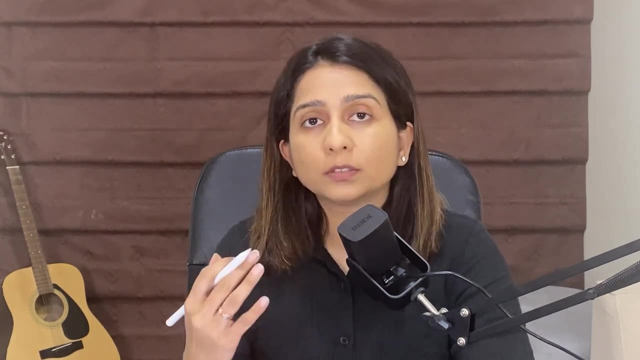 the system and also, it is risky to hold locks on such huge tables for a longer period of time. right, this is one of the huge downsides of this particular approach. how do we solve this? how do we solve this problem? by the way, this problem is also known as long living transactions problem. 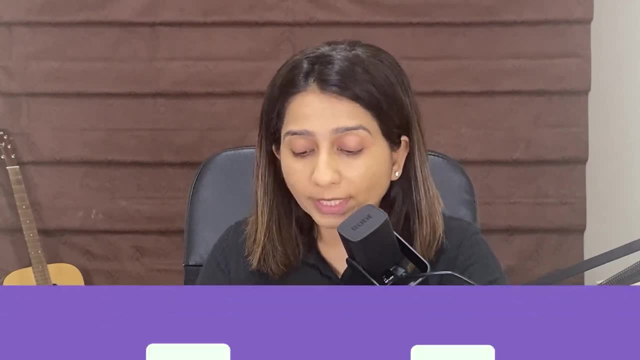 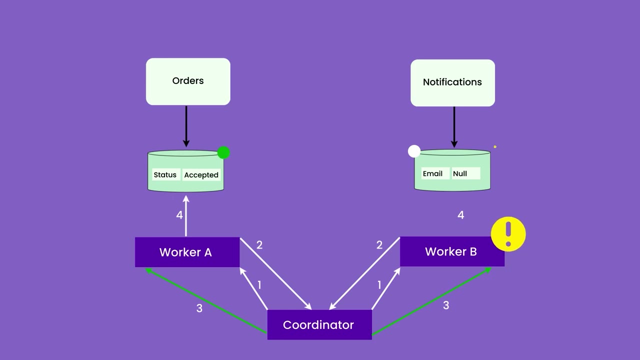 right now. how do we do that? also, when this voting and commit phases are happening, let's say that the voting phase was over and as soon as the commit phase is happening, one of the services goes down or one of the db stops responding or stop accepting connections. 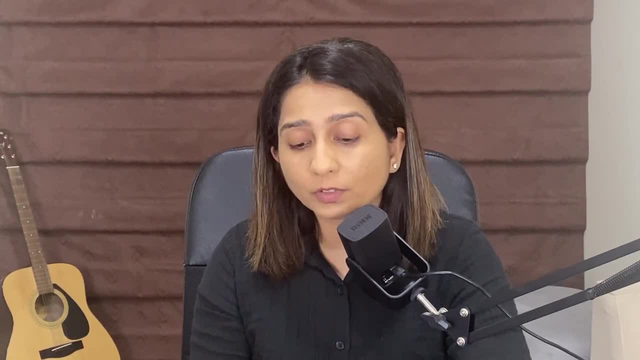 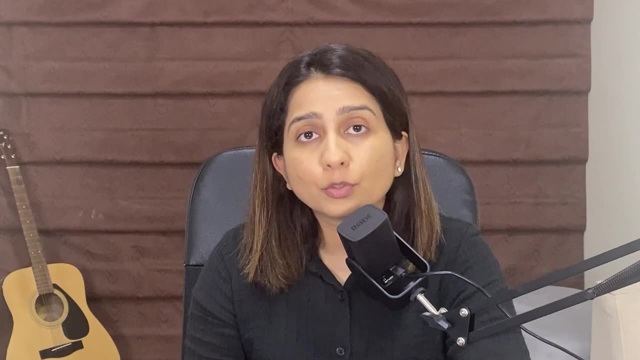 in that case as well, you have the whole failed approach. then you will have to go and release log and you just try the whole thing all over again. what is the solution towards this problem? it's very simple: just don't do it. you don't need to take this approach. it is risky. if you find 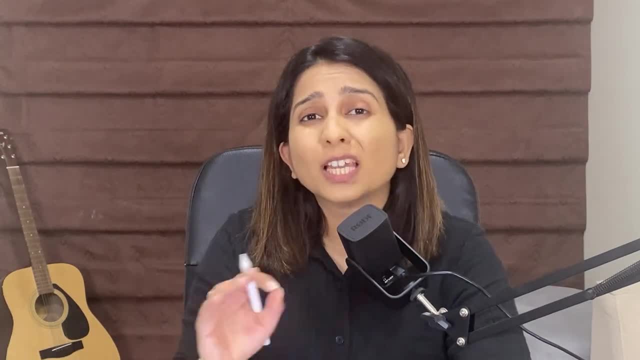 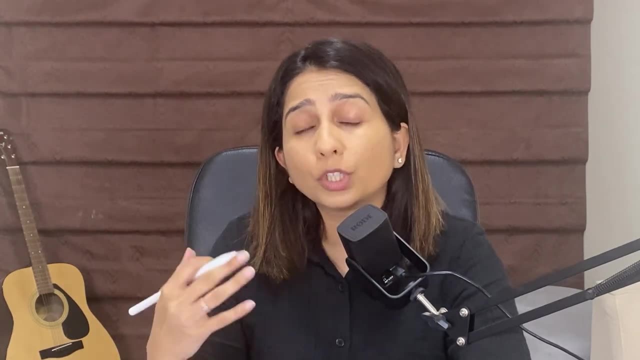 yourself in a situation in your team. we are implementing this approach. if you have less amount of data, it might still be fine for a few days for one feature, but if you see that your data is growing or if you see that you want to do microservices in a right way, then you should not. 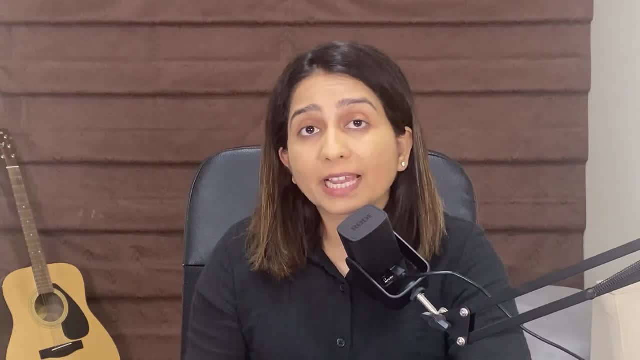 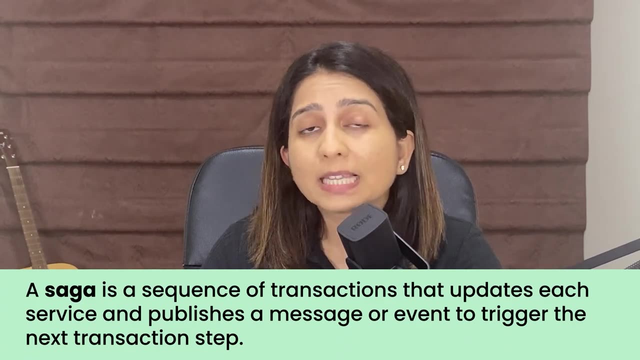 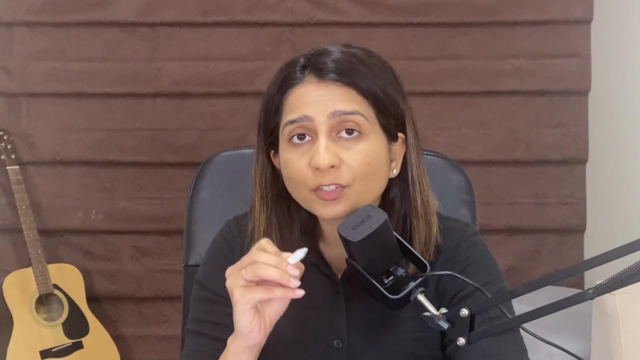 go with this approach at all. now, what is the actual solution? the actual solution in case of microservices is the saga approach, or you must have heard about this term: microservices, sagas saga is nothing. it is a fancy name for an algorithm that solves the problem of updating distributed state in different systems. so let's say that you. 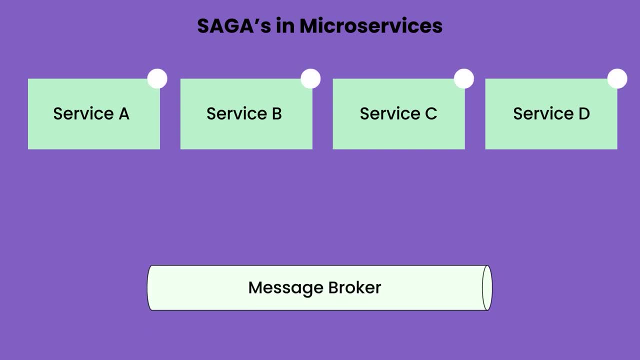 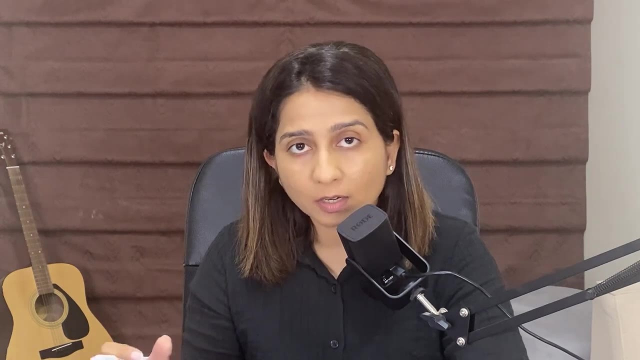 have service a, b, c, d, there is a particular state that is maintained in all the services and it has to be updated at the same time or in the same business flow, in the same business transaction. so any algorithm that helps you achieve this using events is actually saga. saga is much more. 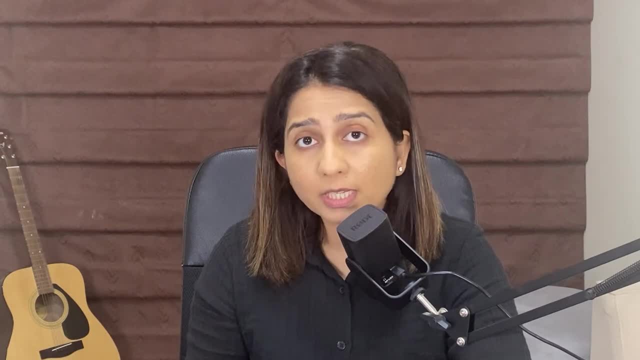 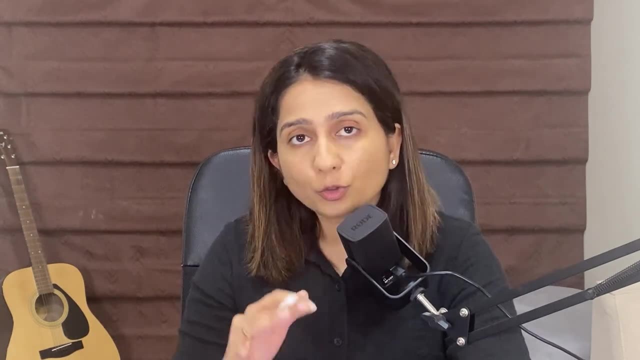 detailed than this. there are different papers written on it. i'm not going into too much details. i'm only trying to help you understand the practical aspect of it, of how it is used in microservices. so let's try to see how transactions take place in sagas. okay, let's say that we have a. 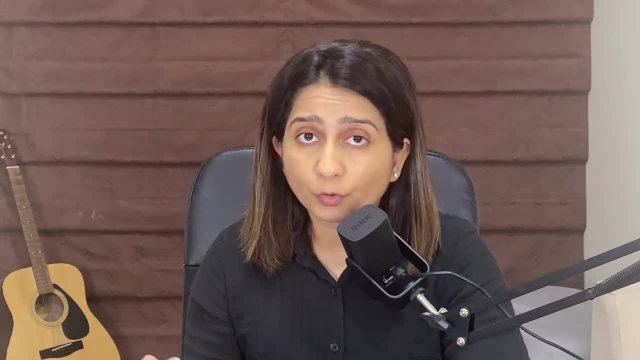 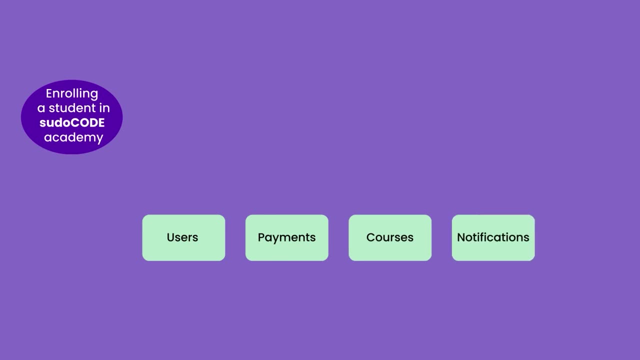 pseudocode academy and we are trying to create an account for a user and trying to assign some courses to them. so how do we do it? we have different services: users, payments, courses and notifications. so what are the steps that we have to do when a new user account is created? 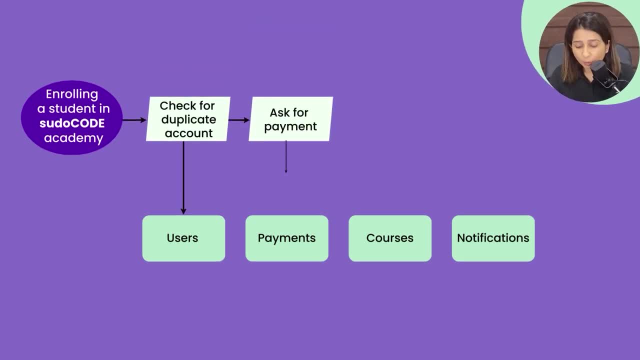 we check for a duplicate account, then we ask for payment. the payment is done. once the payment is done, we create the profile and assign different courses, and once all of that is done, we send the notification to the student or the customer that your account is created. and here are the: 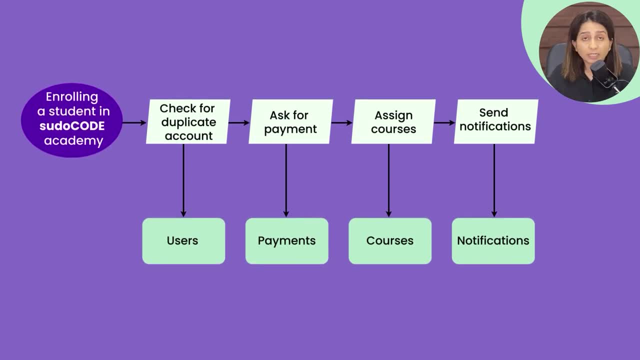 courses that you have been assigned. okay, this all sounds good. now what happens if one of the step fails? let's say that you don't have any duplicate account, but at the step one you don't have a duplicate account, but at the step of the payment it failed. what would you do? or 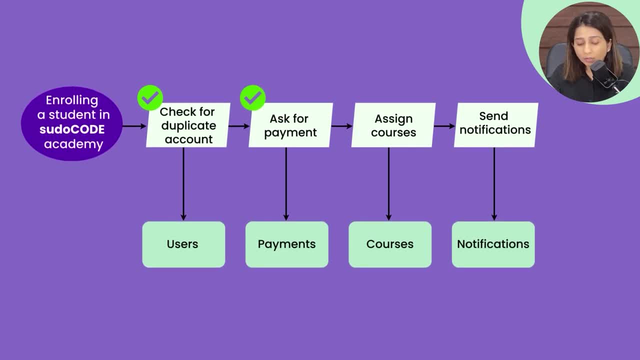 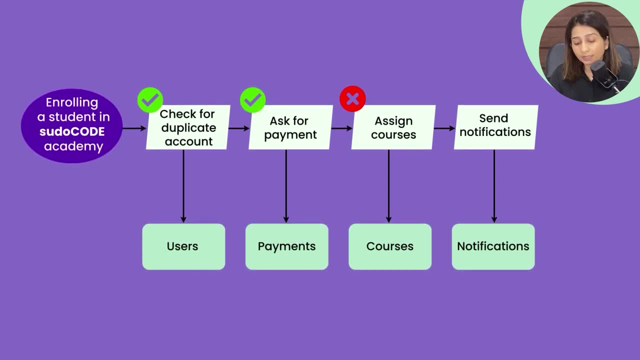 let's say that payment is completed and assignment, of course, is failed. now what do you do? do you go back and not create the account? or do you go back or, like refund the payment? what do you do in this case, because your payment completion has already been done and your assigning to the 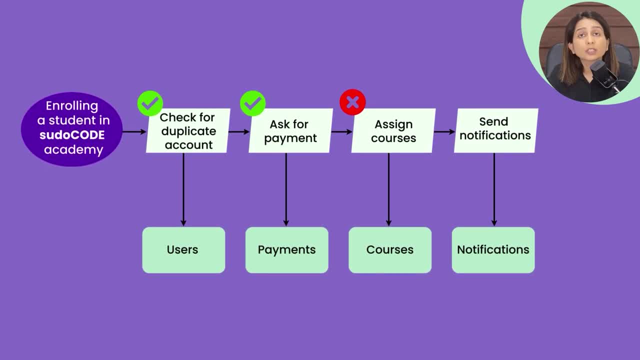 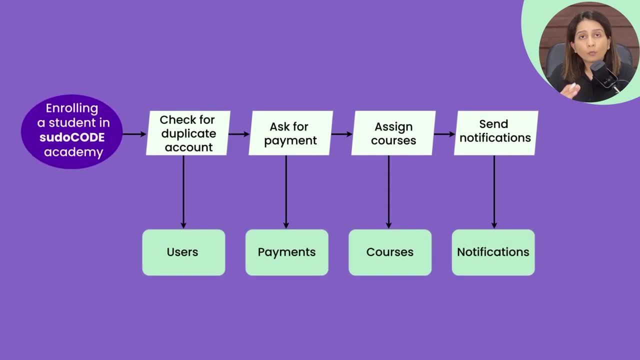 course is still right and you cannot go to the next step. you cannot send the notifications, so they will not get notification that the payment has been made. they will not get the notifications. account has been created right. it is a stuck state, one of the approach that you can take in. 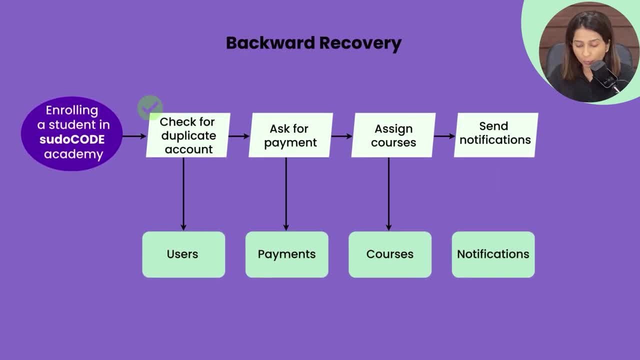 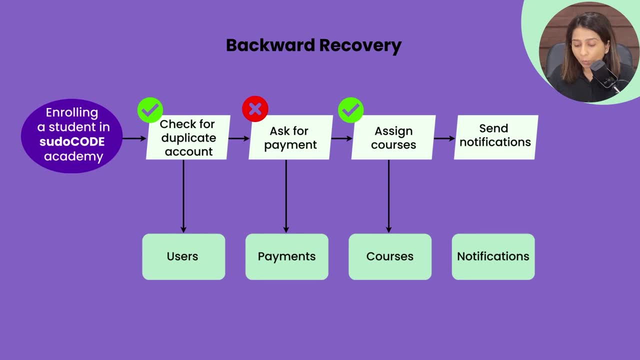 order to solve this is you can have some kind of backward recovery for this. so let's say that your payment failed right and you were able to assign courses, but your payment failed right. what you can do is you can do a backward recovery. you remove the courses, you refund the payment and 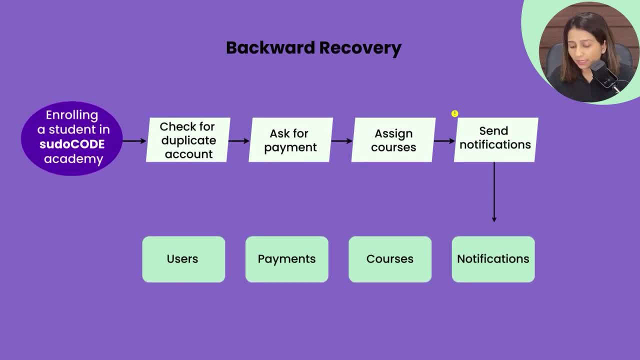 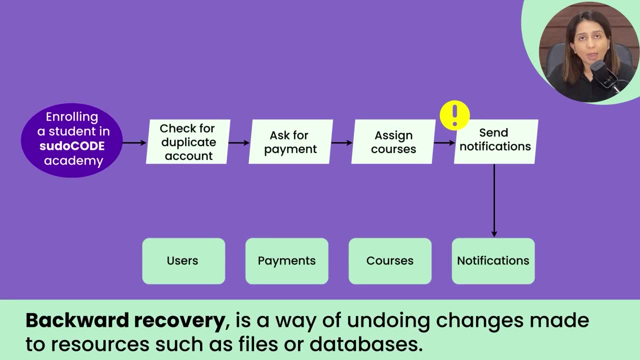 you remove the profile and after that maybe you can send an email that sorry, we couldn't create your account. please try creating it again. okay, this mechanism is called backward recovery, that you repeat the steps that you have already executed, but you do like a compensating backward. 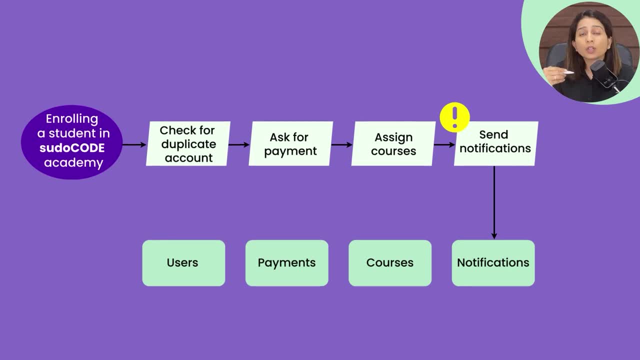 mechanism for it. like you have created the account, remove the account. you have taken the payment, refund the payment you have. instead of sending a success email, send a failure email. that sorry, we couldn't do it right. that is one way of handling it. another way of handling it is that you retry. 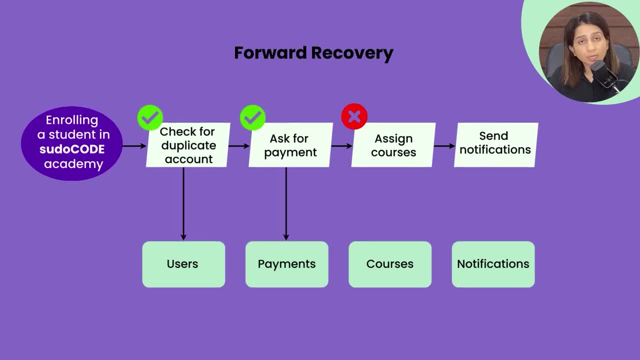 okay, let's say that your payment was successful, but this step failed. what you can do, you can try that step again and continue your transaction. that is another step to make this whole thing successful. this is called forward recovery: that you try to still move forward in the, in the direction, by trying the. 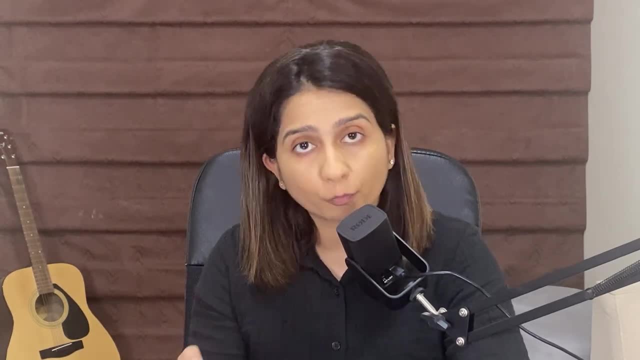 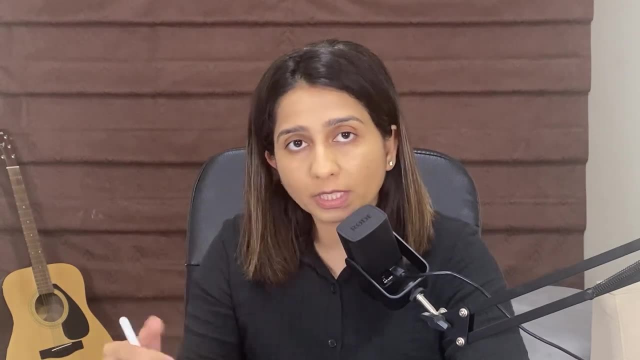 retry of the steps. maybe you can apply the same approach in retrying of payments as well. this approach, where you try to retry, is called forward recovery. instead of going backward, you still try to move forward in the direction of the whole transaction, but you try to retry while moving. 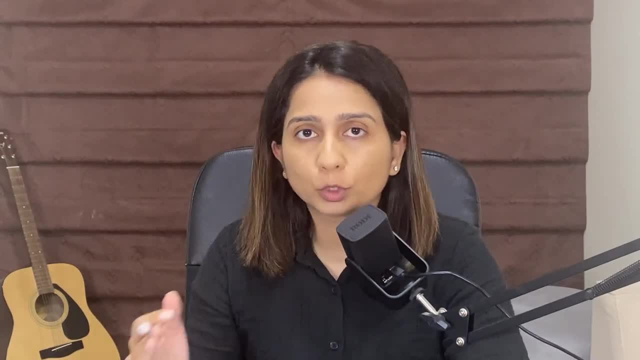 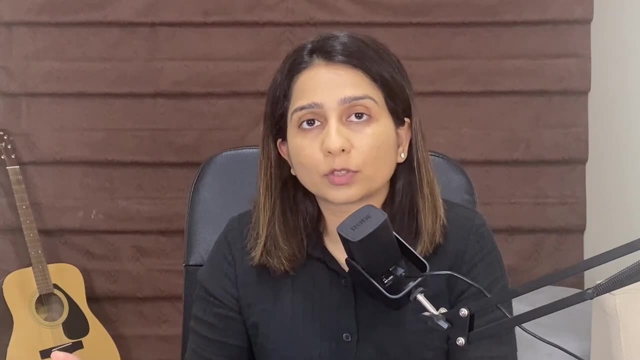 forward. it is completely normal to go with a mixture of both approaches, that you do forward recovery for some steps and you do backward recovery for some steps. now, this was an idea of how saga algorithms are, or how saga transactions are carried out in in microservices. now, when talking about actual implementation, there are two different ways to 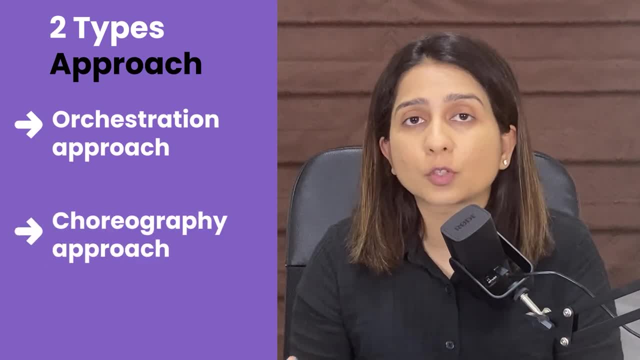 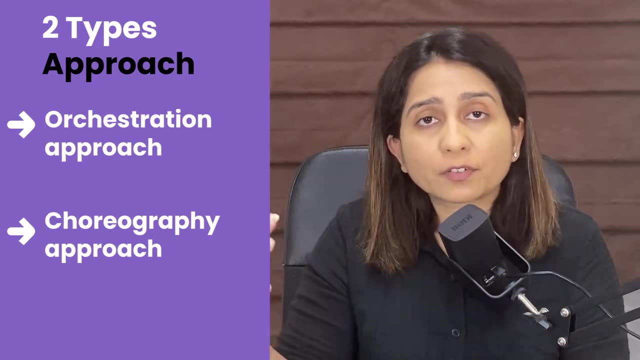 do it. those two approaches are called orchestration and choreography. in terms of microservices, as the name suggests, orchestration is something where there which follows command and control approach. you might have seen in the in the music shows that there is one person who is orchestrating. 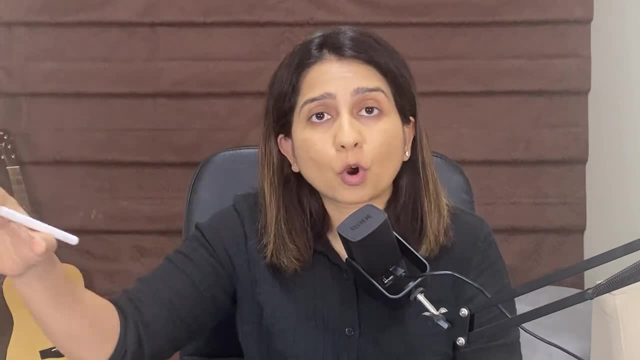 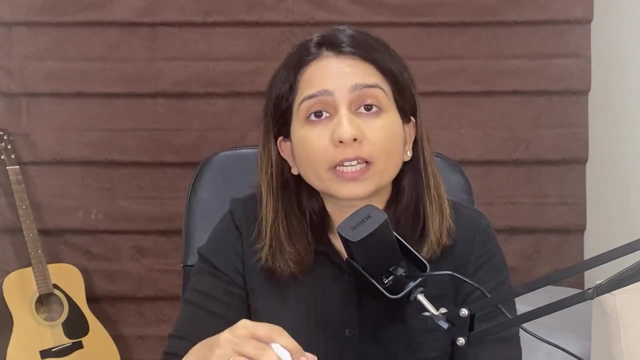 the whole show. so they have a command and control over who plays what, when certain groups stop and certain groups starts playing, and so on. right. so command and control is the type of architecture or the type of problem solving approach that's taken in orchestration, whereas choreography is. 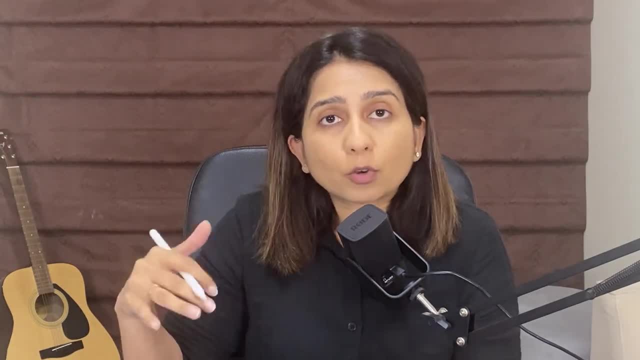 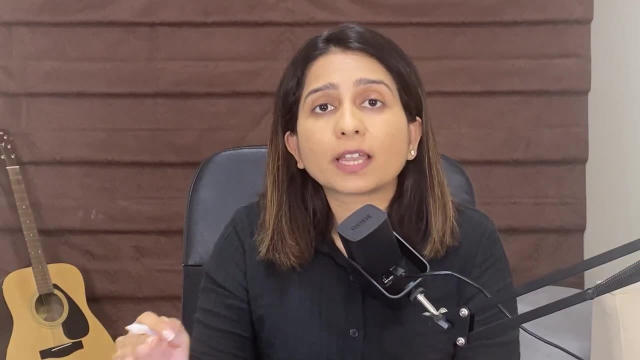 an approach of trust. but verify, so you. there is a choreographer who tries to teach the dancers or the or the performance, like how the whole show is going to look like. but it verifies by practice and rehearsals that, okay, you will do fine. and at the time of the show itself there is no choreographer. 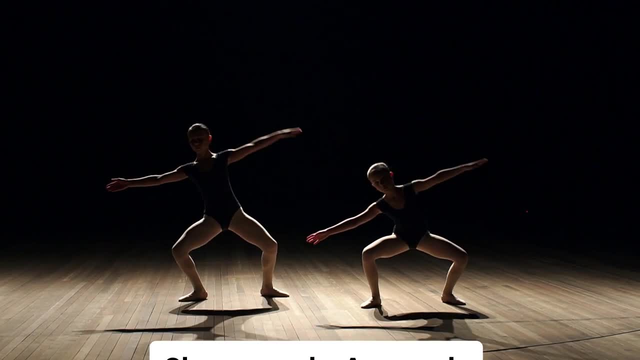 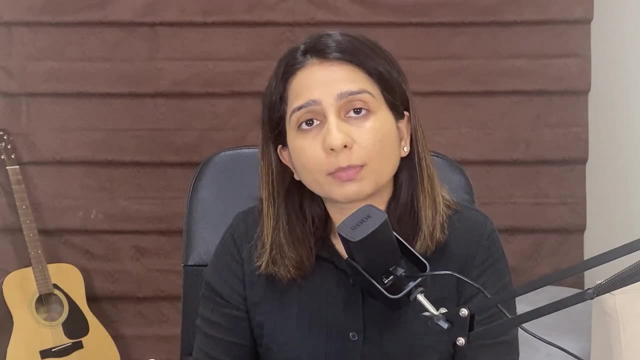 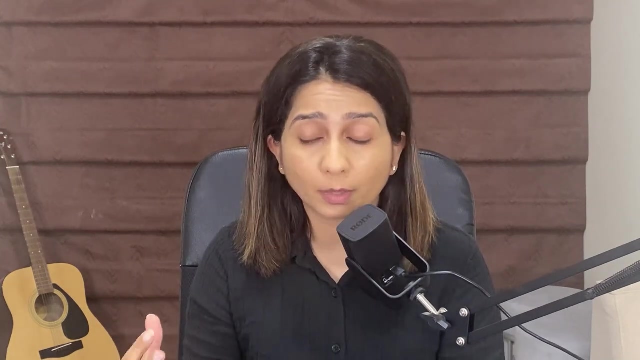 to handle anything. the, the dancers or the performers handle everything on their own right. so these are the two fundamental differences between these two approaches. you will see when how sagas are implemented. the same approach is applied to those solutions as well. now let's say what? how does the orchestration approach would 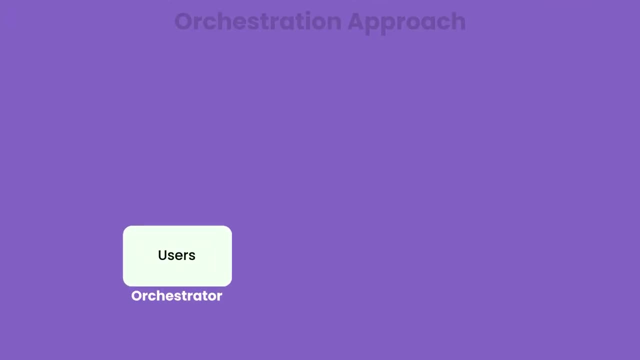 look like. so in this case, your user service is going to act as an orchestrator. the user service is going to ask course- a service to pair the user with with the courses, and also user service is going to create the user account. it will take the payment from the payments and once that, 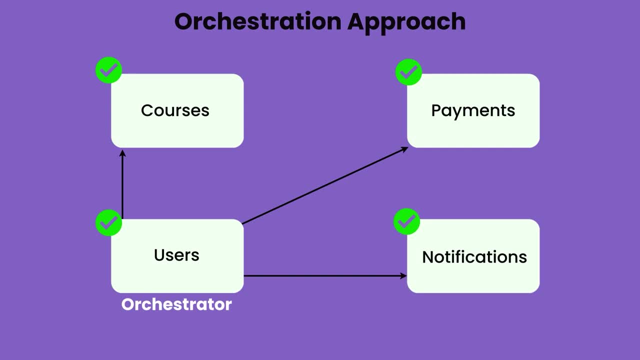 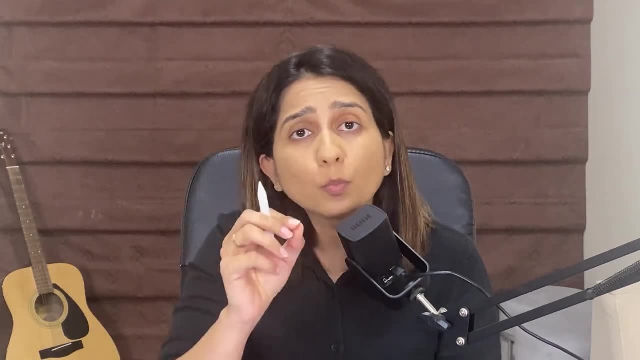 is successful, it will send the email. it will ask the notification services to send email. so basically, user service has all the command and control. it is talking to different services and telling them what to do. like you course a service, please spare the courses. please take the payment. 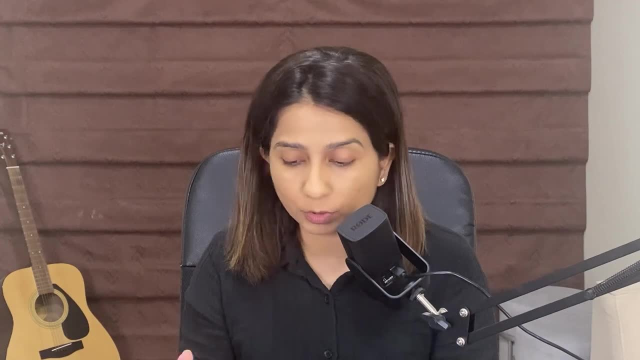 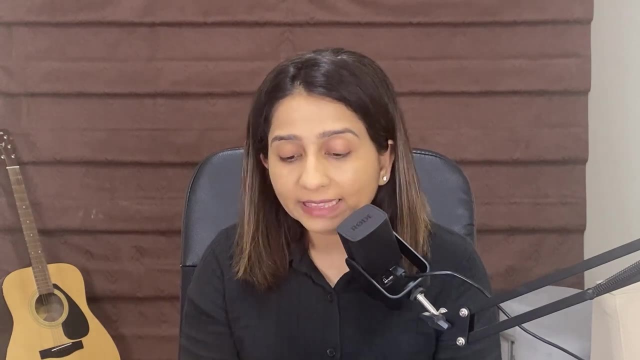 and please send the email right. so this is how an orchestration approach looks like. now how does choreography looks like? choreography is just like event-based architecture all over again. in this case, there is no controller, there is no orchestrator. all the services are independent and they only. 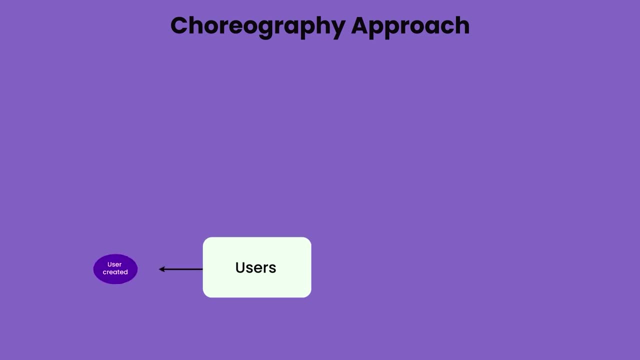 depend on the events. so user service emits user created event. course service reacts to that user created event. it takes the that event and maybe pairs some courses to that user. so the courses service is going to emit the event that user is paired with. the courses payment service might consume that event to take the. 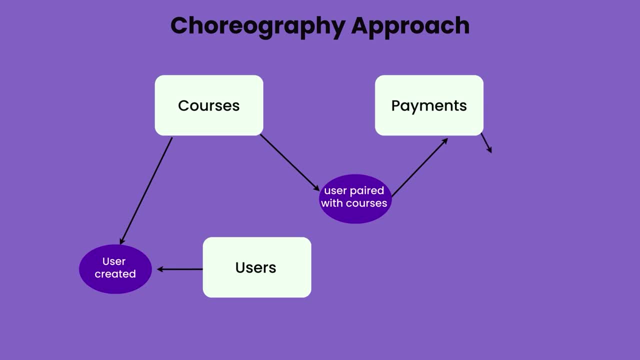 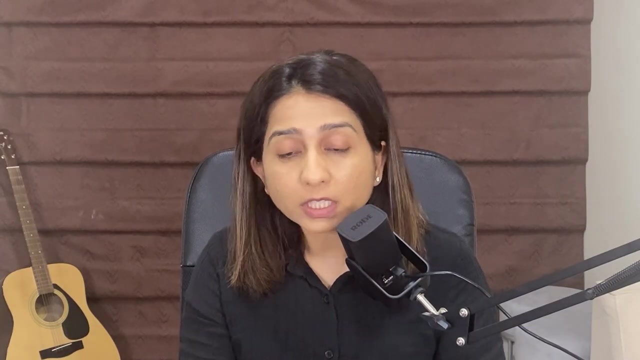 payment for those courses. once payment service has done that, it emits the event payment done and then notification service consumes that event and then sends an event of send email or actually sends the email, right? so you see here none of these services are acting as a commander, none of these services have control. all these services are just emitting. 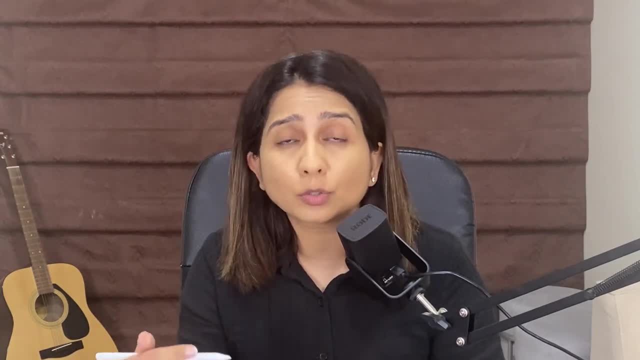 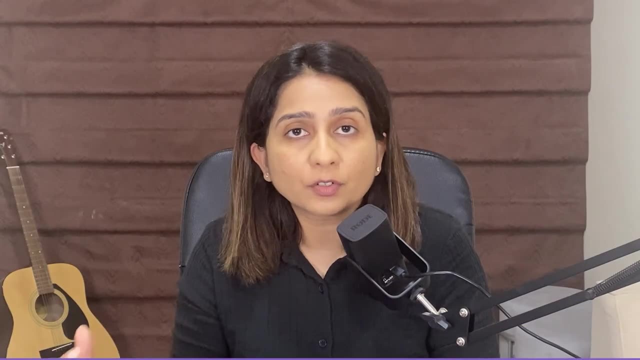 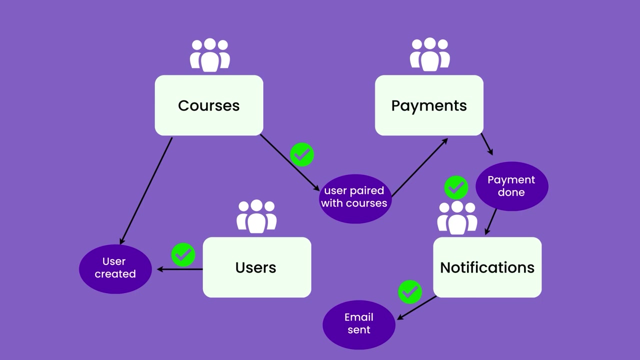 the events and all the different other services are reacting to those events to complete the whole business flow. right now, how does this get implemented in real world scenarios? so all these services would be owned by different teams and when a certain business transaction or a business flow has to be implemented, these teams will come together to align on the contracts of. 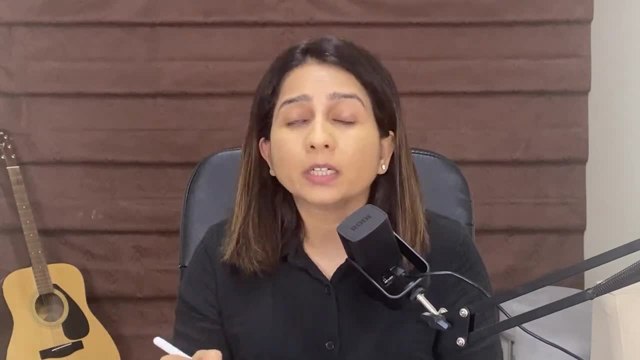 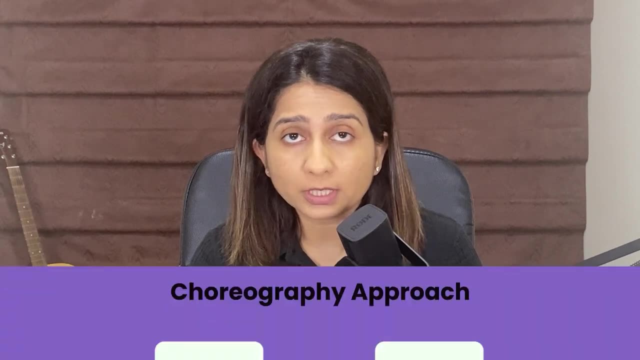 these events and what would happen in the reaction to these events in order to implement the whole flow. now, both these approaches have their pros and cons. one of the con of choreography approach is that whenever something goes wrong, you need to find out where it went wrong. it might be courses. 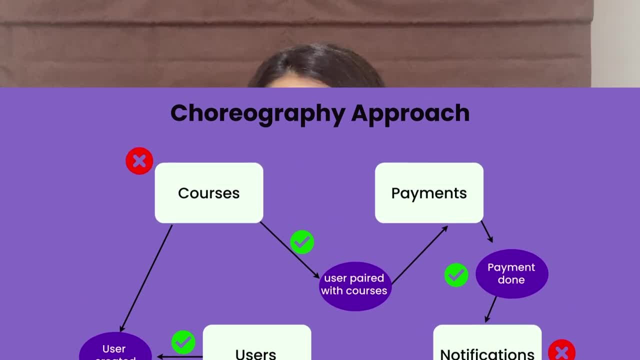 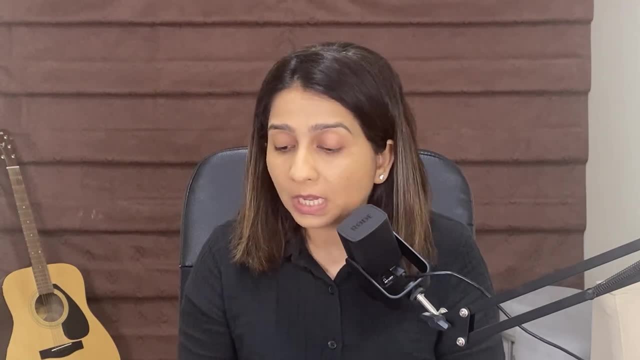 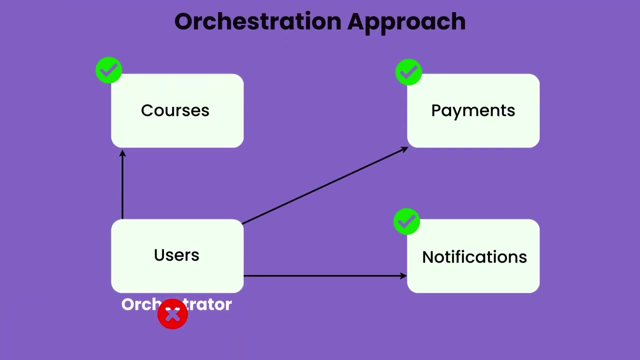 service, or it might be notification service, or it might be some glitches in the data that is sent in the events. so you need to have very good observability and monitoring in your system to figure that problem out. in case of orchestration or orchestrated services, you generally have one orchestrator, so you might find the origin of the problems. 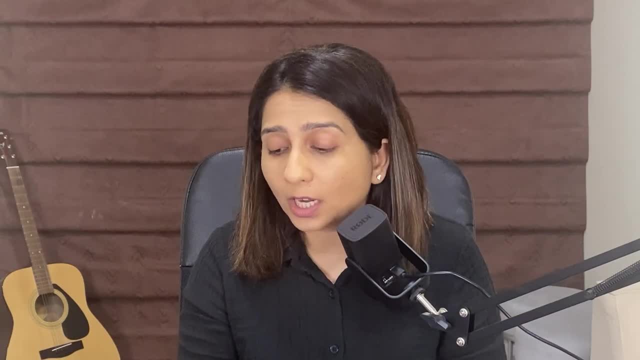 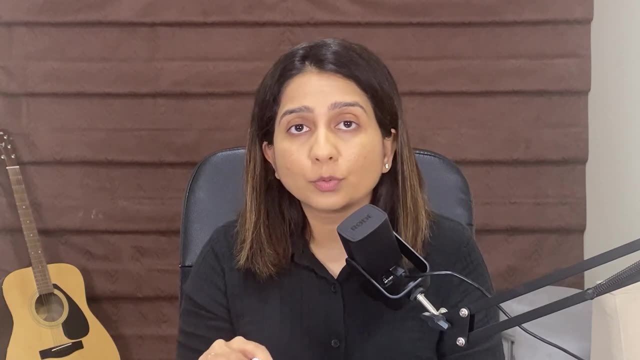 starting from that particular service. but even in this case it might happen that the problem is in some downstream service and it might take you some time to figure that out. one of the approaches that is used in order to debug issues in in both these approaches is correlation id. whenever these. 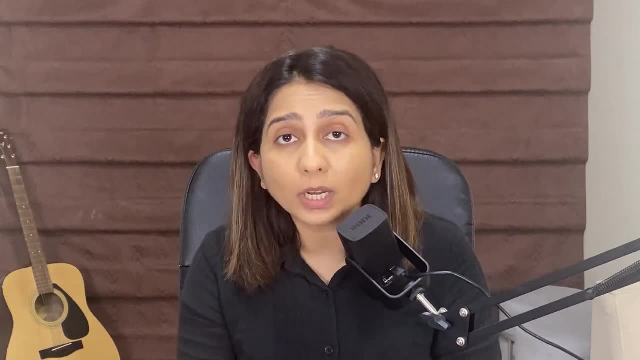 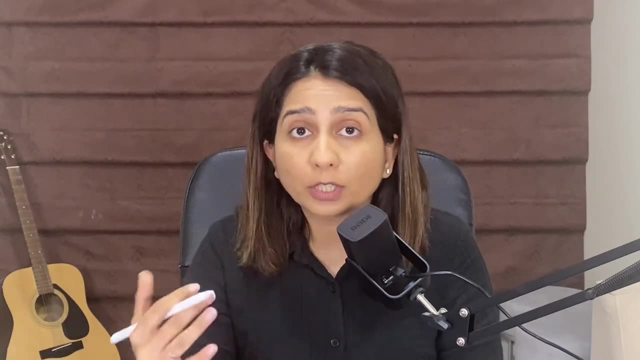 services are producing some kind of logs, they all might use one particular id or a request id to emit the logs. that is known as correlation id. it's again a deep concept, but you can go and google it up so that correlation id will actually help you to do that, because it's known as correlation id. it's. again a deep concept, but you can go and google it up so that correlation id will actually help you to do the stuff that you're doing. and that way you can kind of make the situation better, which is see all the transaction across different services, like when which event happened in which service. 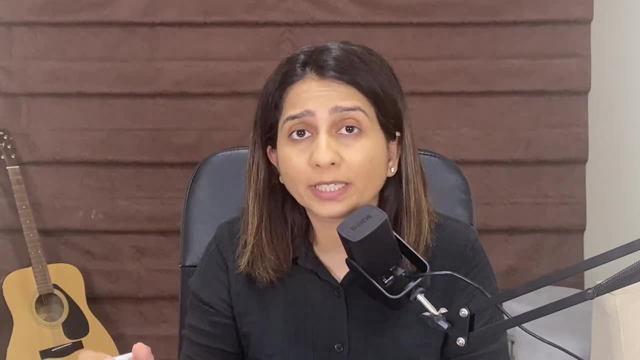 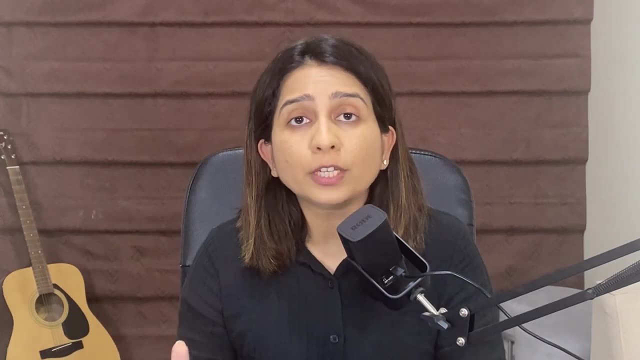 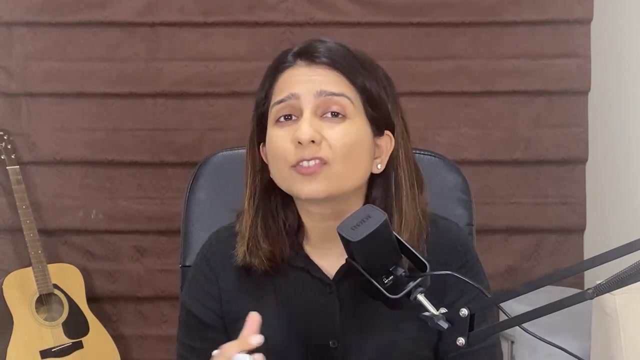 how a particular service reacted to that particular correlation id and you can pinpoint the culprit service which failed to fulfill the event or fulfill the transaction. now how do you choose? when do you have to go with, uh, distributed transactions, like we discussed that you shouldn't do it. or when should you go with sagas? right, in general, it is not recommended to go with. 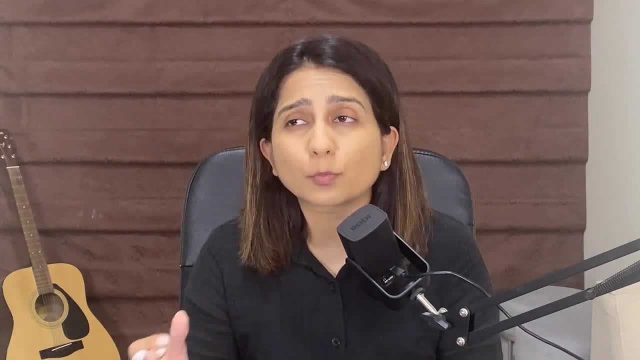 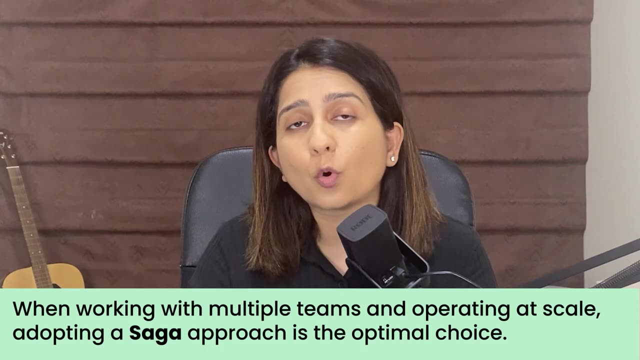 distributed transactions. but again, if you are just bootstrapping or you have small services, small data sets, you can actually try it out for some time. but whenever you have scale and you have a lot of teams, it is recommended to go with the sagas, depending on your services and the architecture.